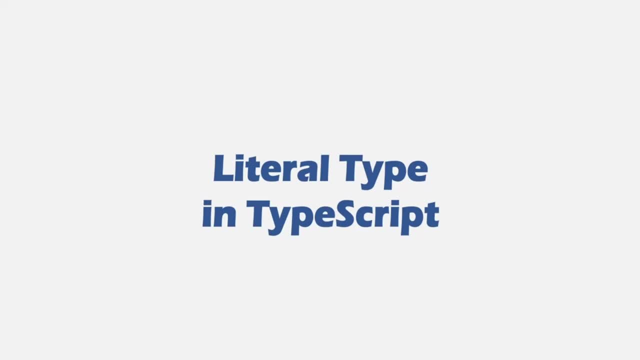 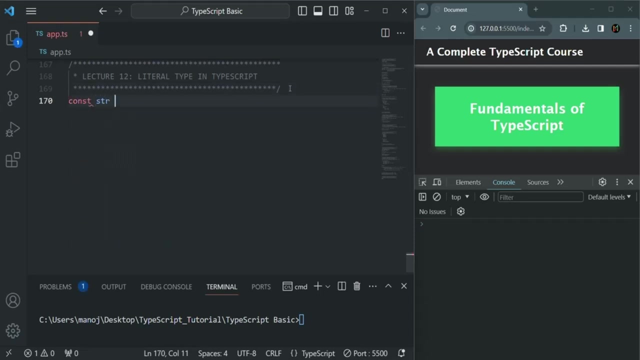 we don't just tell what type of value we want to store in the variable, but we tell exactly what value we want to store in a variable. Let's try to understand it with a practical example Here. if I go ahead and if I create a constant variable, let's say str and to: 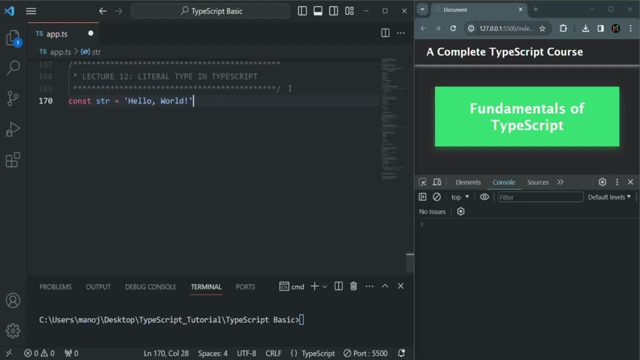 this: if I assign hello world and if I hover over this str variable, you will notice that its type is this string value: hello world. Now, internally this hello world is nothing but a string value. But if we check the type of this str variable, it is not saying string. 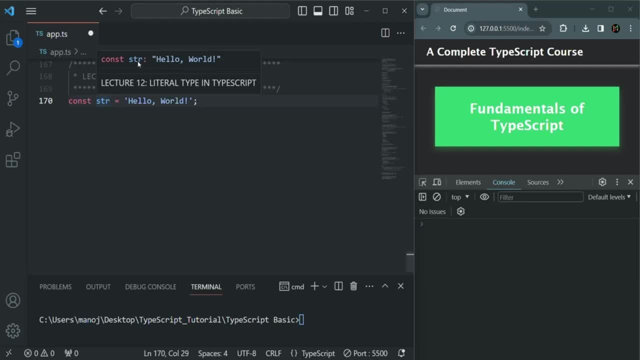 It is saying: hello world, the value which we have assigned to this str. And this is what a literal type is. A literal type simply means the value which we have assigned to a variable. it will act as a type for that variable, In this case the value. 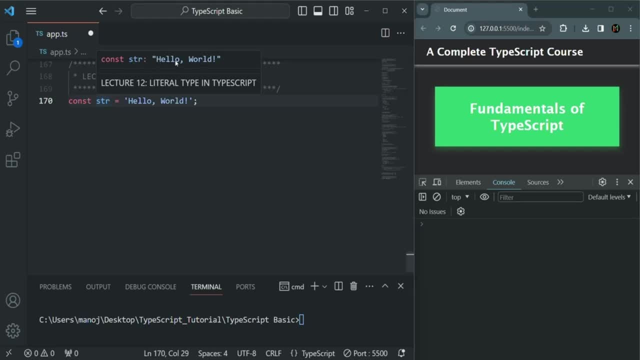 which we have assigned to this str variable is hello world. So this hello world is the type for this str variable And this is a literal type. If I create another variable using let keyword- let's say str2, and here also if I assign a string value to it, maybe. 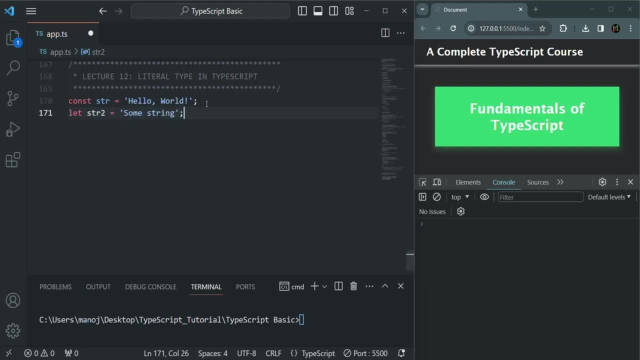 some string. and if I hover over this str2 variable, here the type is string, Here the type is not the value which we have assigned to it, Here the type is string. But in case of this str variable the type is hello world, the value which we have assigned to it. And 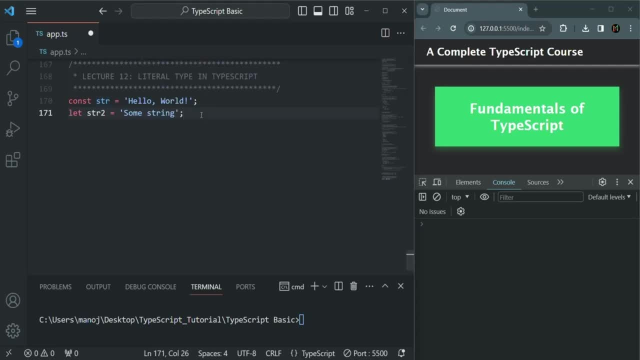 this is what is called as literal type. Using a literal type, we don't just tell what type of value we want to store in a variable. Let's try to understand literal type with another example. So what I am going to do is I am going to create a function and I will simply call this function maybe roleMessage. 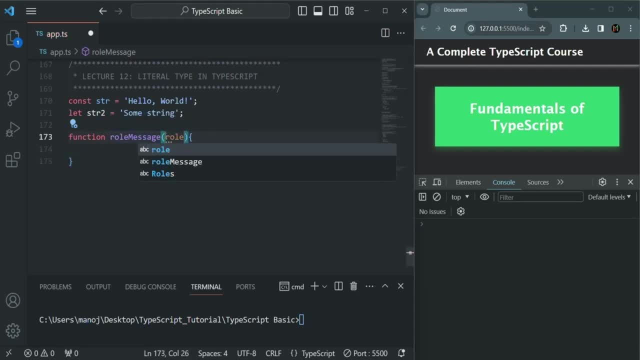 And this function is, let's say, going to take a role parameter and for now, let's specify its type as string. Now, inside this function, I am going to write a switch statement and to this switch we will pass the value in the role. 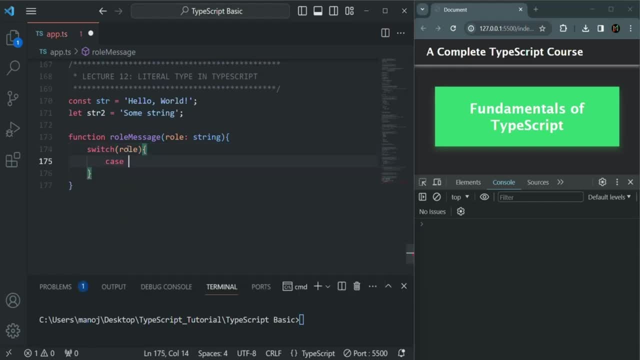 And then we are going to write some cases. So case first is going to be admin. So if the case is admin, in that case we want to return a message. or let's say, we want to log a message in the console saying that you have admin permission on this site. Okay, and then 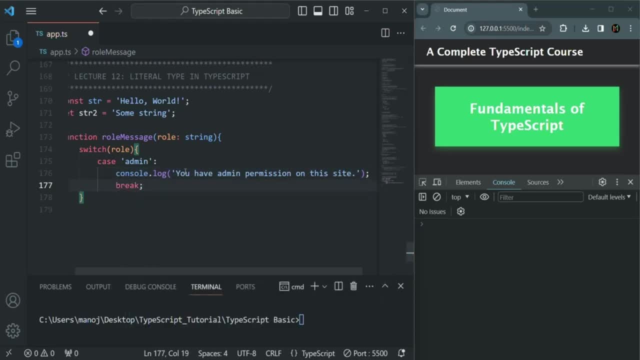 let's break from here. Then, in the same way, let's add another case. This time let's say the case is read. Again, we are going to write a consolelog statement And there we will say: you have read permission on this site. Again, let's break from here And let's write another case. 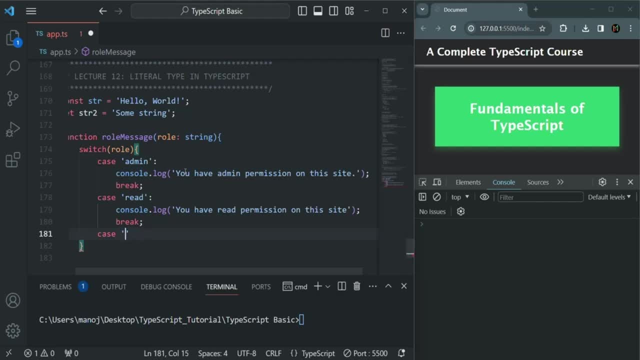 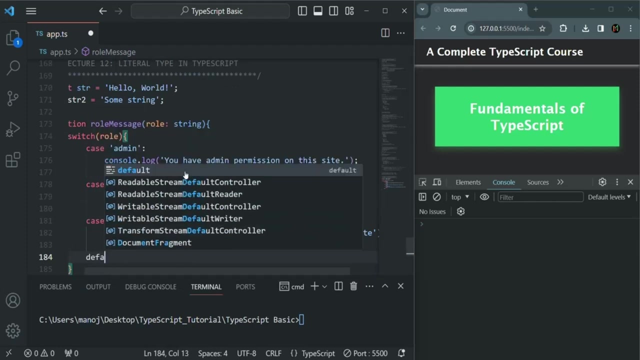 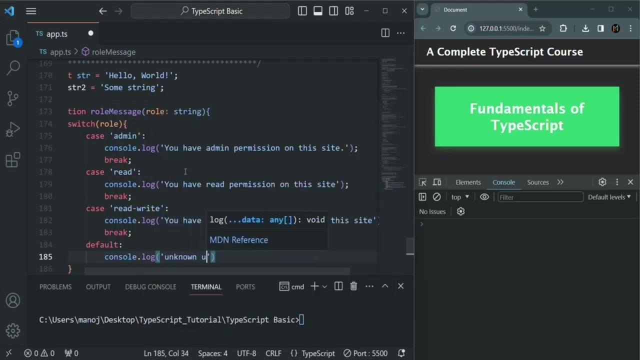 And here let's say permission is read write, So read hyphen write. In that case we want to say you have read write permission. Okay, And then we are going to add a default case, And for default case we will simply say unknown. 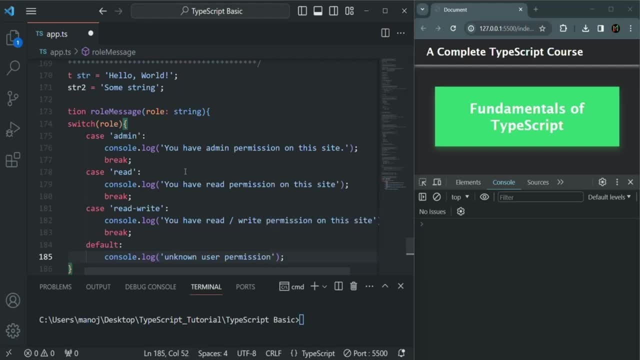 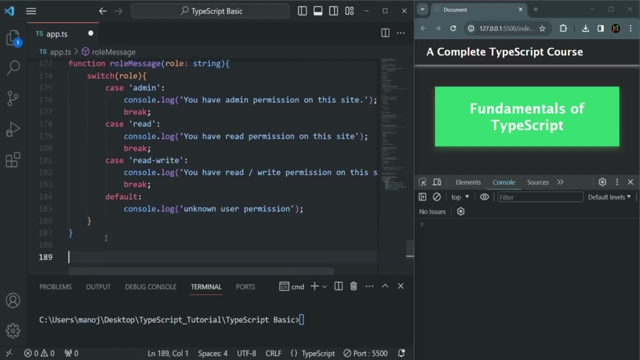 user permission. All right Now, when we are going to call this role message function, let's call it here. In that case, we need to pass a value for this role parameter. So currently we can pass any string value. So if we pass admin, let's save the changes. Let's compile this appts. 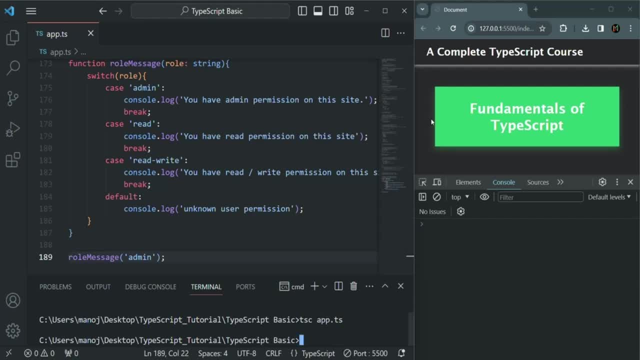 file And if we refresh the page, you will notice that it logs this message: You have admin permission on this site. If I pass some other string value, let's say read, write, Okay, Let's see if the changes- let's compile this appts file again. And now it says you have. 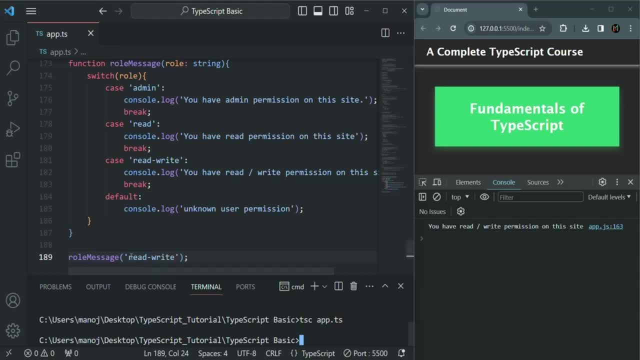 read: write permission on this site. So it is working as expected. If I pass any other value, for example some random string like abc, if we save the changes And if I compile this appts again, you see it says unknown user permission. so it is working as expected. 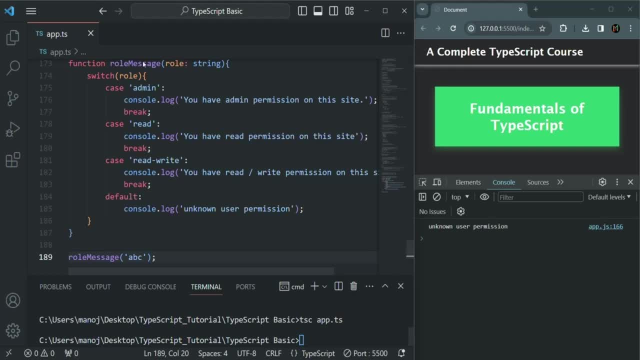 But what we want is when this function gets called for, this role parameter. we only want user to either pass admin or read, or read write. no other string value should be allowed for this role parameter. currently, since we have specified its type as string, we can pass any string. 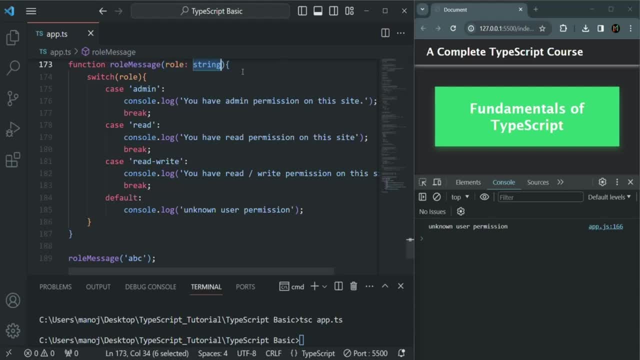 value. but for this role parameter we need a specific string value. it can be either admin, read or read, write, and that we can achieve using literal type. so here what we can say is, for this role parameter the type should be either admin, so the value should be either admin. then we will use this union, then. 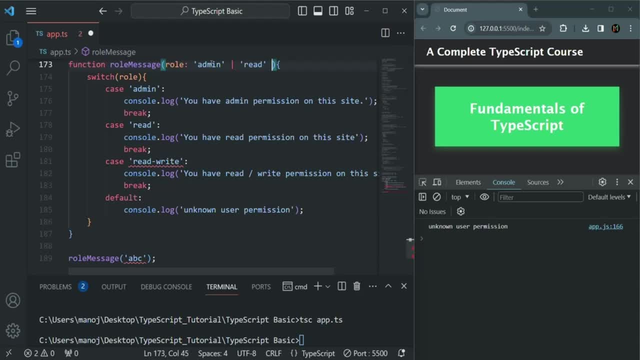 we will specify another value, let's say read, then we will use union and then read write. so these are the only three values which we want to accept for this role parameter. so here, if I hover over this role parameter, its type, it does not say string, as you can see, it does not say string. as you can see, it does not. 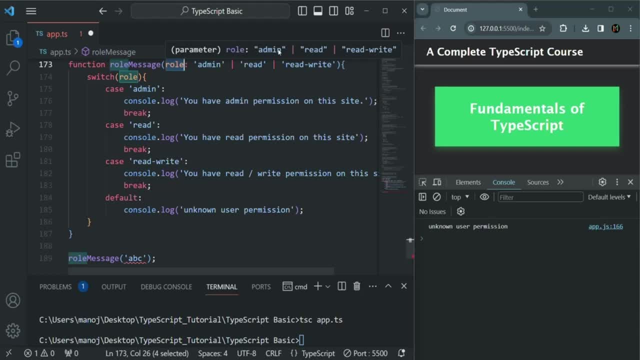 say its type is string, instead its type is this okay, and this is a literal type. so this is basically a combination of literal type as well as union type. so here we are using some literal values and then we are also using union type using this pipe symbol. so now, here you can see, we already have an error, if I 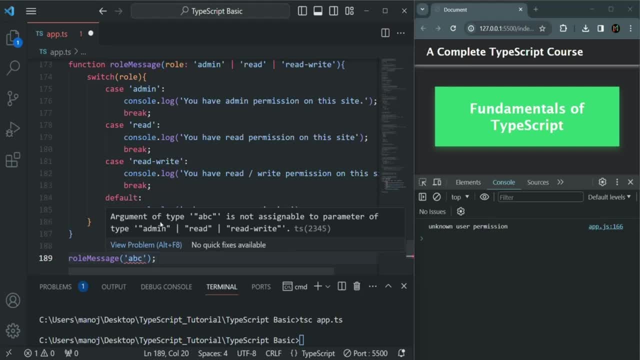 try to pass ABC we have an error, because you can see the error message that ABC tells us that we have an error and the type is admin, union, read, union, read, write. if I specify admin here, in that case that value will be allowed. but if I don't specify admin, if I specify some other string value, you see we have an. 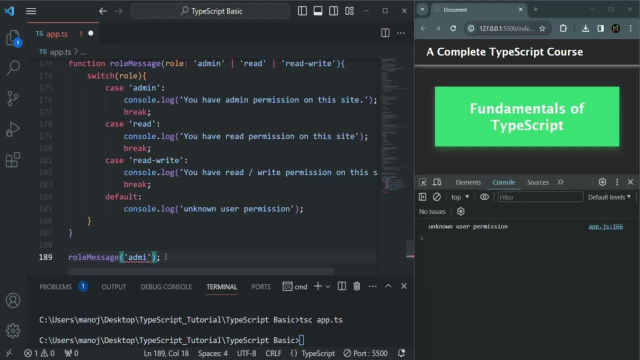 error. so a literal type basically tells what exact value we are going to accept for a variable or for a function parameter. I hope the literal type is correct. so let's pass admin here, let's save the changes and let's compile this application. and now you can see here. we have this message, you have admin.